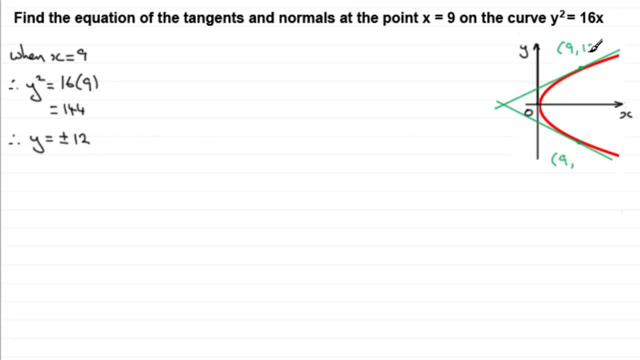 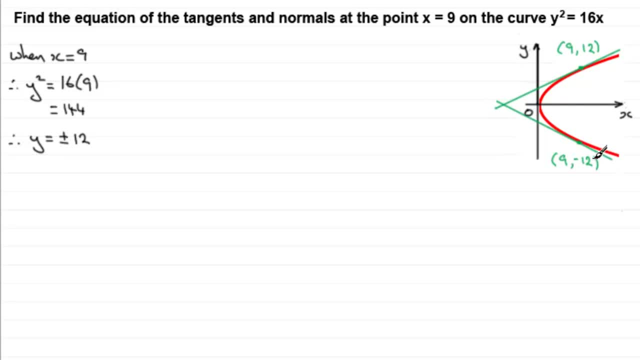 Well being straight lines, we need to get the gradients of these lines, which will be found by getting the gradient of the curve at the point where x equals 9.. Now, when it comes to working out the gradient, we need to differentiate our equation for 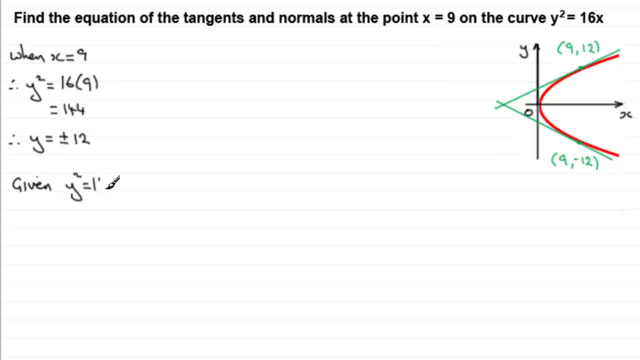 the curve. Now, when it comes to working out the gradient, we need to differentiate our equation for the curve. that y squared equals 16x, and there's two ways that we can go about differentiating this. we can either use implicit differentiation or we could make y the subject and just differentiate it that. 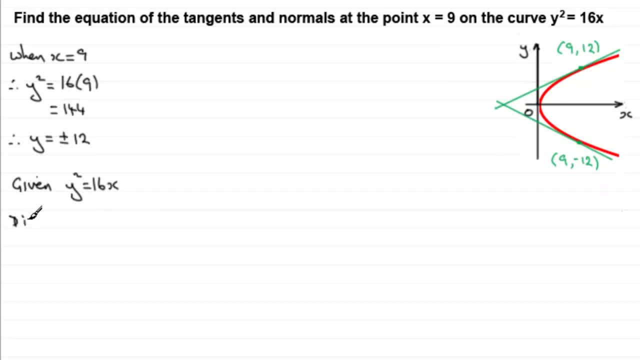 way i'm going to go. first of all, though, for differentiating implicitly, so i'm going to write differentiate with respect to x, and, assuming that you're familiar with implicit differentiation. if not, you can always go on my website. there's plenty of tutorials on implicit differentiation. 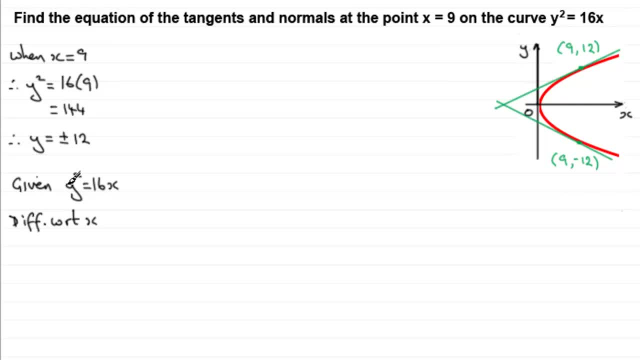 but assuming that you're okay with that, differentiate y squared with respect to x, we get 2y. dy by dx. and then if we differentiate 16x with respect to x, we just have 16, and then, if we divide both sides by 2y, we end up with, therefore, dy by dx. 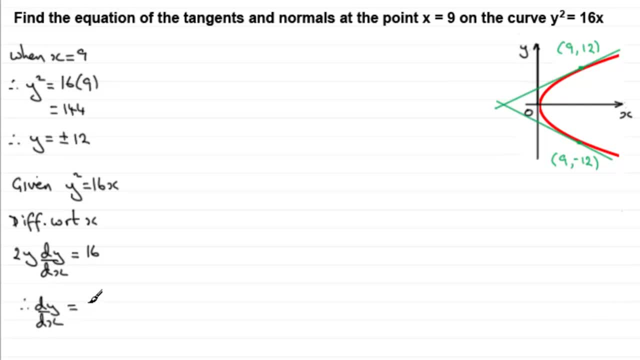 dx equals 16 divided by 2, so that's going to be 8, and then it'll be over y. i'll call that equation one. that's one way, then that we could differentiate this, so let's just line that off there. so what was the other way? i'll do it in blue, okay, just to. 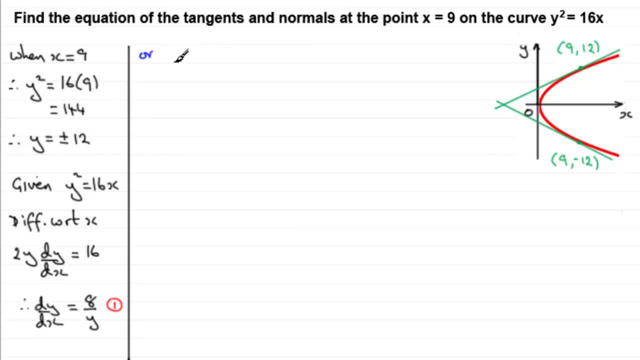 separate it. all we could have done then that make y the subject. we could have square rooted both sides. that would give us y equals 4 root x. y equals 4 times the square root of x. but i'm going to write the square root of x as 4x to the power half, so it would 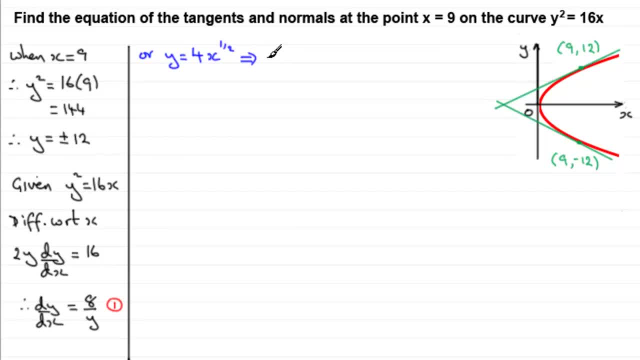 follow from that result that, if we were to differentiate this with respect to x, dy by dx would be equal to four times a half, which is two drop the power by one, so it'd be x to the power minus a half. in other words, 2 over the square root of x, 2 over x to the half, 2 over the root of x. 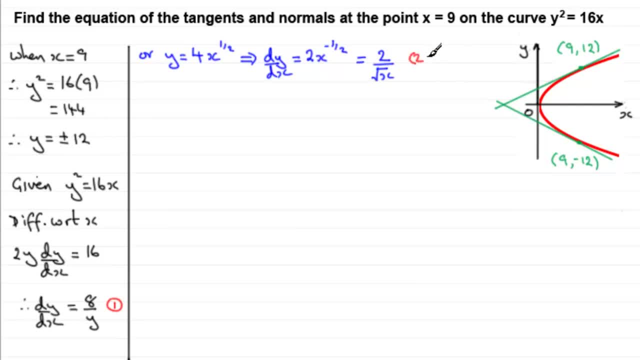 and i'd call that the other version, let's call it 2.. so to work out the gradient, then, of these tangents, i would need to just say, for instance, if i'm going to use this version here, i could say: when y equals 12, 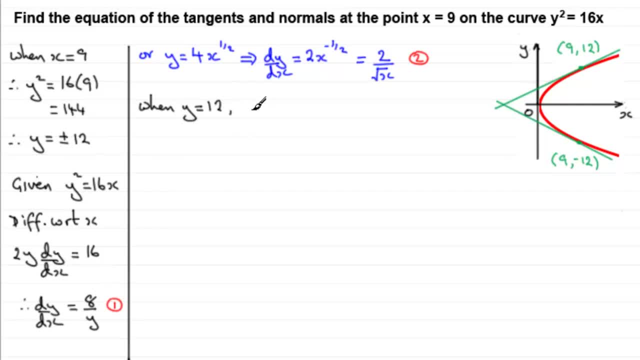 because it depends on y. dy by dx. or we could just say: 1 gives okay. that dy by dx equals 8 over 12.. 8 over 12 cancels. you can divide top and bottom by 4 and you get two thirds. or if you used 2, let's just again do that in blue. you could say that when: 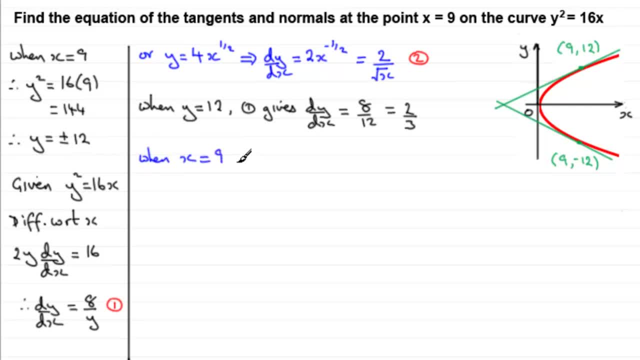 x equals 9. all right, then equation 2 gives dy by dx equal to 2 over the square root of x, x being 9, 2 over root 9, square root of 9 then will be 3.. two thirds, so you've got a gradient there of two thirds. 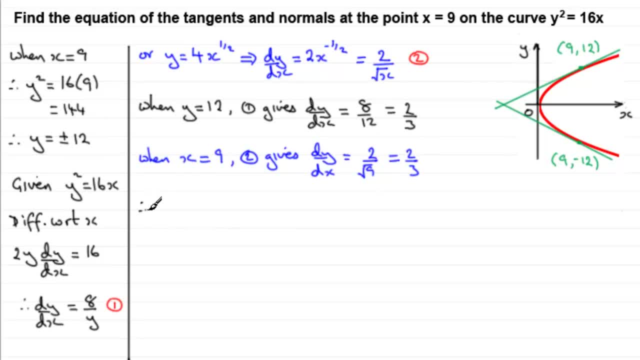 so either way, we can therefore get the equation of the tangent. so, therefore, the equation of the tangent. just write a header here, okay, and we'll say what point we're looking at. and that's the point where x is 9 and the corresponding y value is 12.. 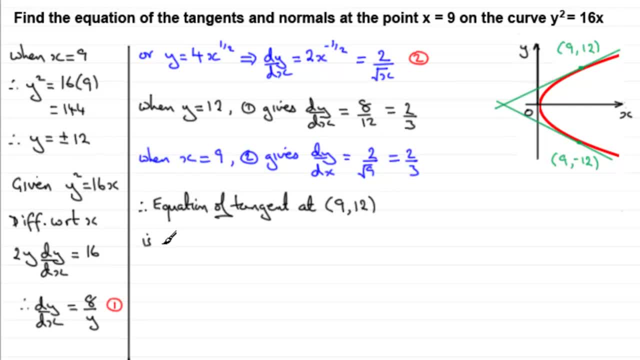 what's it going to be well, if we use the standard formula, y minus y 1 equals m bracket x minus x 1, then it will be y minus y 1. being 12 equals the gradient m at two thirds multiplied by x minus x 1, x minus 9.. 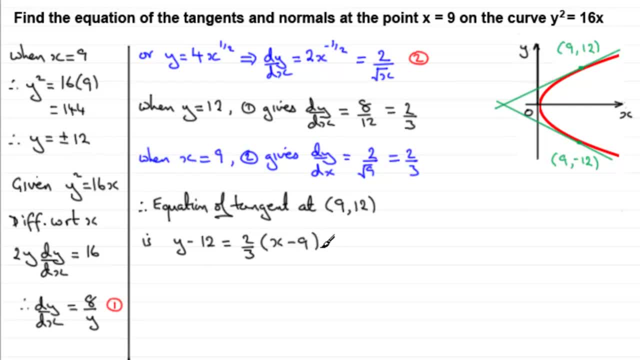 now i'll leave it up to you to rearrange it, if you want, into any particular format, but essentially that's the equation, then, of this tangent through here, and when it comes to working out what the equation of the normal is, then i've got to. now, in a general equation, we want to obviously get the gradient of the normal. 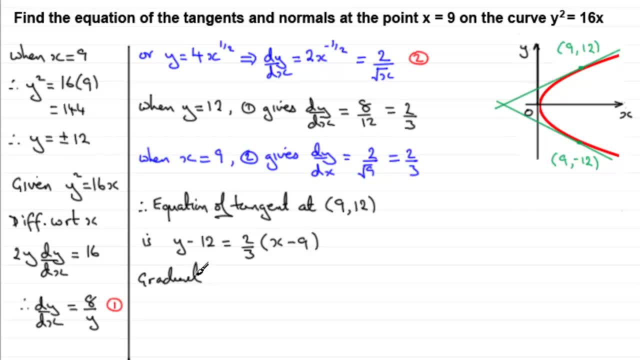 and that gradient of the normal, let's just write it in here: gradient of normal. okay, it's going to be the reciprocal, the negative reciprocal, of what it was when x was equal to 9 or y was equal to 12. same gradient: it was two thirds then for the tangent, so now it's going to. 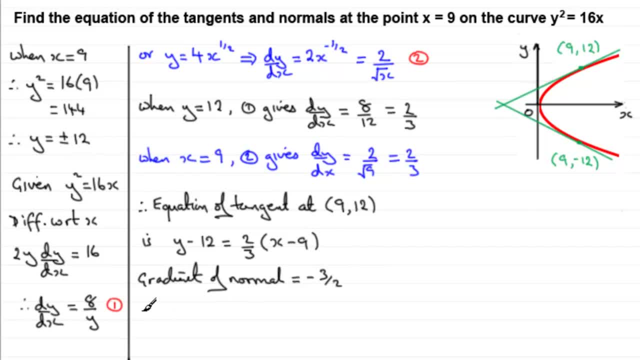 be equal to minus 3 over 2. we can similarly work out the equation of the normal- all right, the normal at 9: 12- just by using y minus y1. again, y1 being 12 equals m, the gradient minus 3 over 2, in this case. 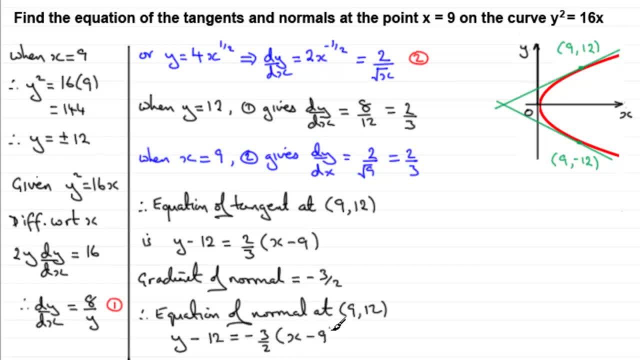 multiplied by x minus x1, so it'd be x minus 9. so that would give us the equation of this normal here. let's just draw that in. it's going to look something most probably like that. okay, carrying on up there, being at right angles, obviously to the tangent. 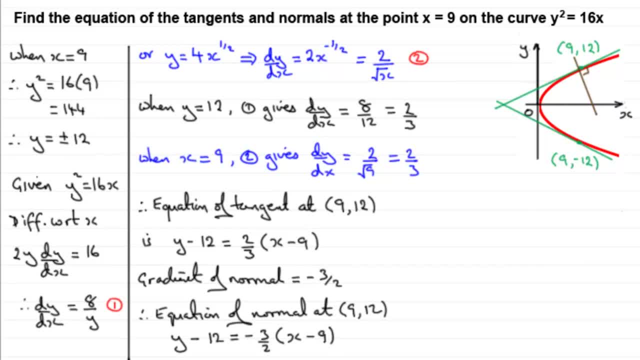 well, if we want to get the equation of the normal here at 9 minus 12 and the equation of the tangent, then basically we've got to do much the same kind of thing again. and so if we just come down here we can see that when x equals 9, we know that y would equal minus 12. when we're looking at this, 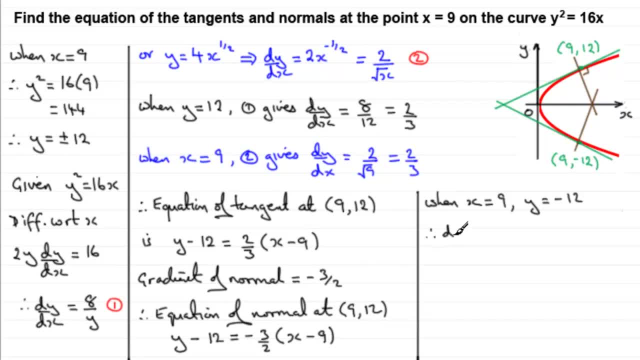 point here. So when it comes to the gradient of the tangent dy by dx, we can use either 1 or 2, doesn't matter. but you'll find that that gradient, if we use, say, 1, becomes 8 divided by minus 12 and that's going to give us a gradient of minus two-thirds. It really shouldn't come as any.